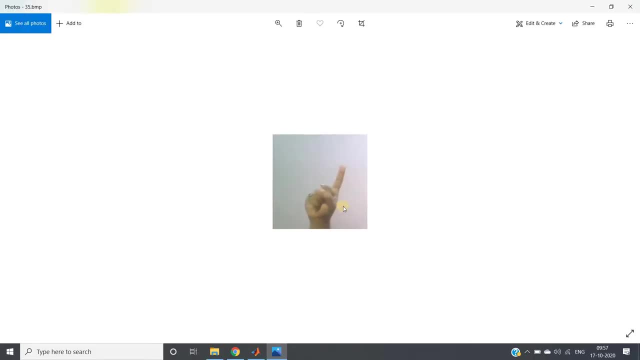 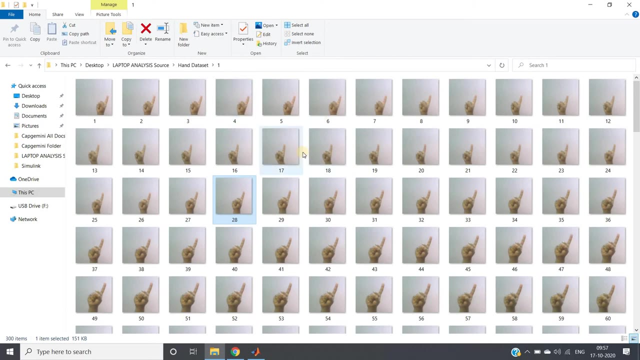 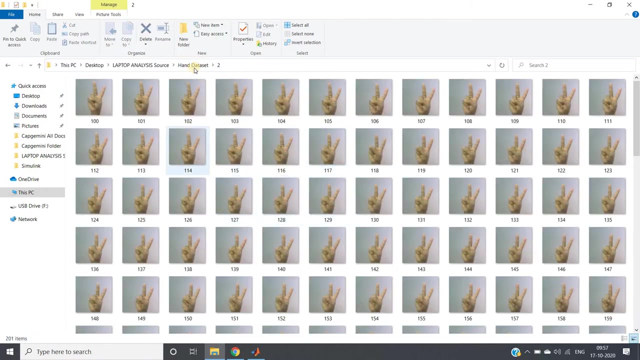 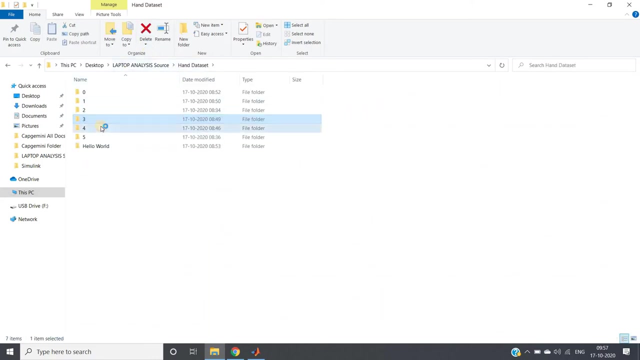 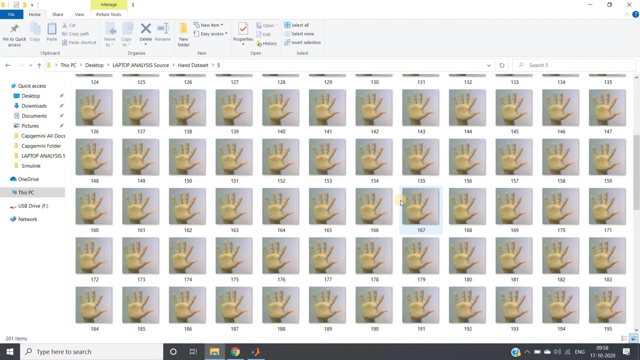 So this is the image of showing one. Similarly, here, many images I have taken. Okay, all the images are resized, Because for Alex Nate you cannot give any size image. I will be discussing that Right. So then, for 2, similarly fingers to showing images are present. for 3, images of 3 are present. for 4, images of 4 are present and for 5, images of 5 are present. Okay, so this is quite huge data set, And if you want to take each photo by mobile camera, then it is going to be present. Okay, so this is quite huge data set. 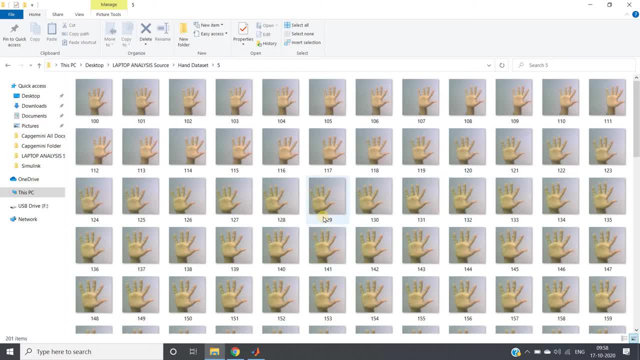 be a very much difficult job- okay, not difficult, boring job, i can say so. i'll be showing how we can do this job easily. also, that is data set collection, data collection part. but first let me show you the actual code. okay, so all of my images are stored in which directory? see in this. 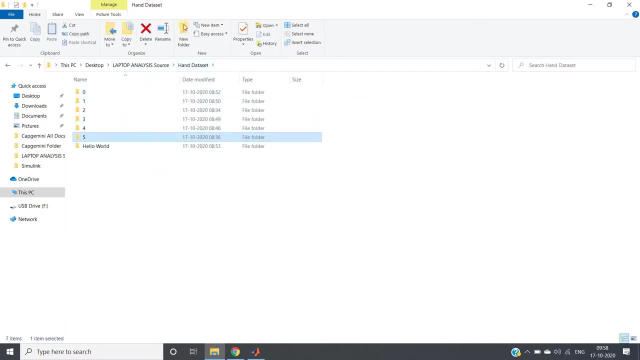 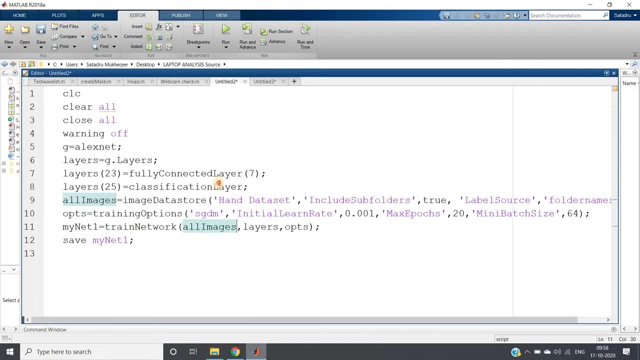 folder, hand data set. all the images are stored. okay, so my main data store is hand i. hand data set. okay, hand data set right. so here is the code: clc- clear or closure warning of g equal to alex net. i am taking the alex net right and then i am extracting the layers and layer of 20, third layer. 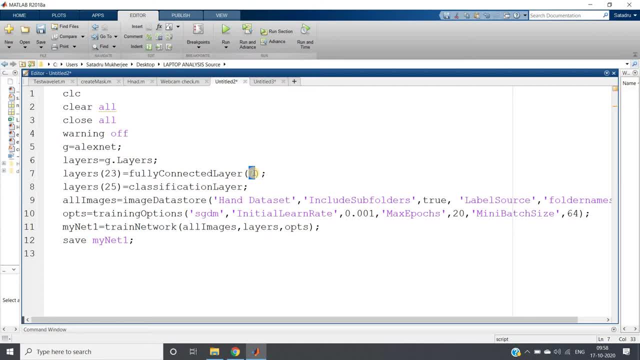 in that i have to specify how many outputs possible. classes are there in my classification model. here you can see there are seven output possible, see zero, one, two, three, four, five and so seven total, right? so here i have written seven. like: suppose you want to have classification only. 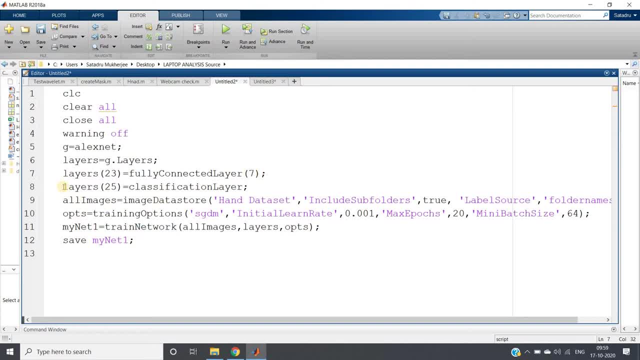 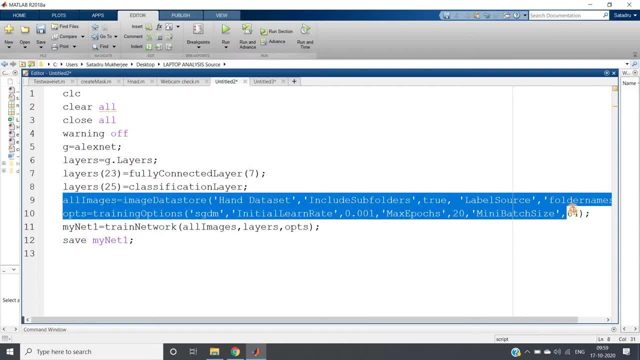 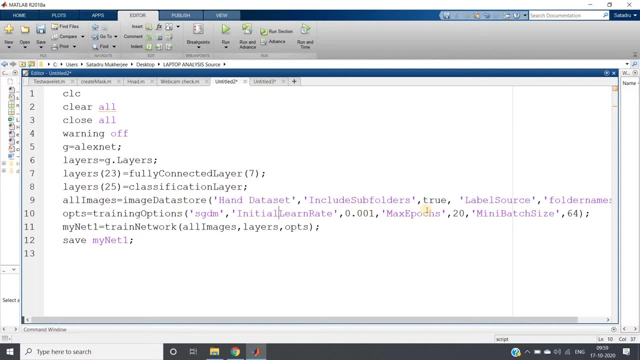 in between two classes, then you have to specify this as two and layer of 25 you have to mention as classification layer and rest part. just, i am specifying the sgdm, that is, stochastic gradient. descent: okay. initial learning rate. maximum number of epochs: okay. mini batch size: okay, because 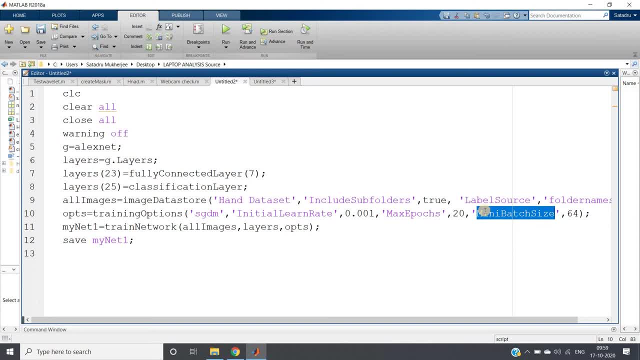 minimal, meaning we are using minimum size. because we are using minimum size, because we are using it is optimized than batch gradient descent or normal gradient descent. okay, and then i am training my network using all images and what is all images? basically all images, basically image data store. we are using hand data set. see our actual folder where all the sub folders of images. 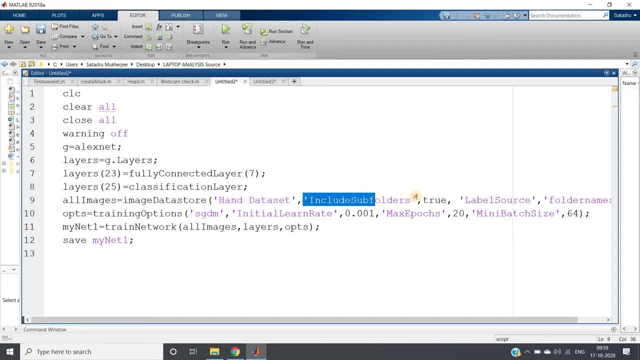 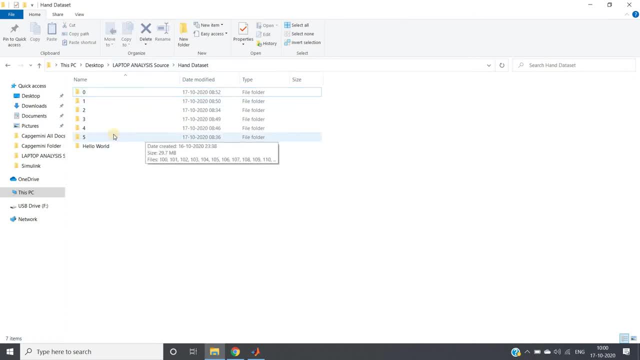 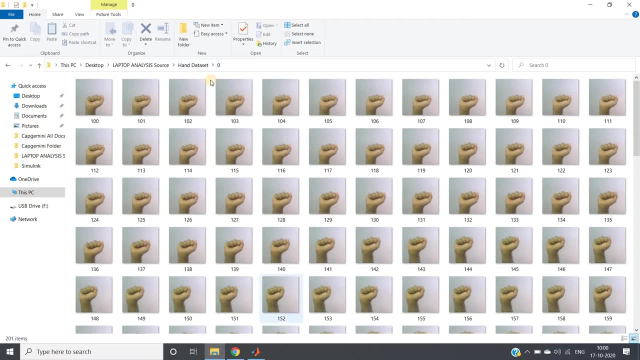 are present. that was hand data set, so i am specifying the name. include sub folders. okay, because you can see inside hand data set, different sub folders are present and our images, uh, name. okay, classification name is basically the folder name. see inside zero folder folder with name zero, images of zero are present, right, so i am writing here. level source is: 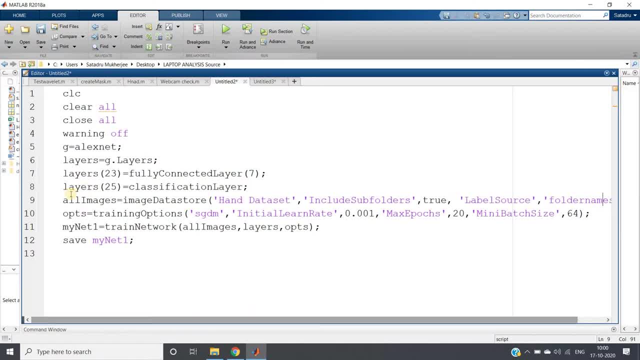 folder name. so, because folder name is going to be my level source and then once you train the model, each time it will take very huge time. so what we can do, we can save the network. okay, save my net one here. you can see in the current directory. here it is. 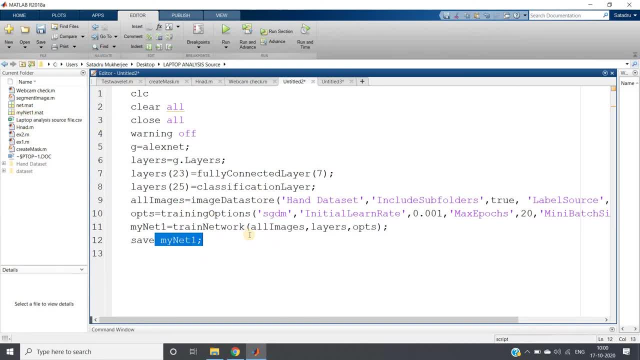 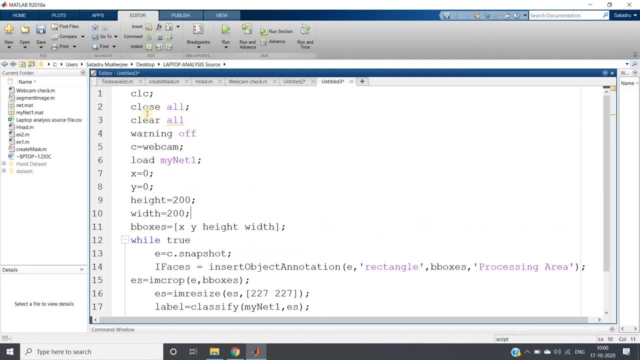 or see my net one dot mac, so later we can use directly this one. we no need to train the model each time, okay, and then here comes the testing part. so clc, clear proposal, warning off, okay, c equal to webcam. i am loading my uh pre-trained model, my net one, whatever we have. 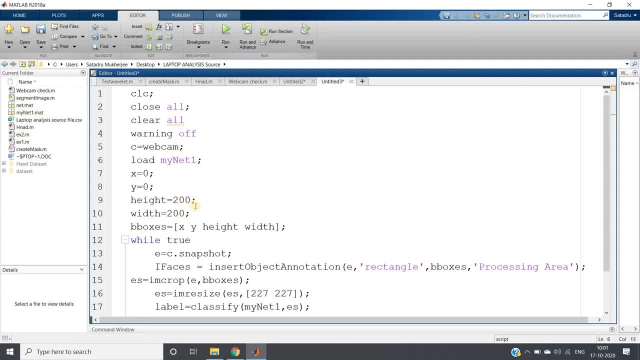 created here using transfer learning. and then what i am doing? i am creating one particular area highlight. i want to highlight one particular area. if you want to count number of hands, then you need to take your hand in that particular area only. that is our processing area. we can say, okay, x equal to. 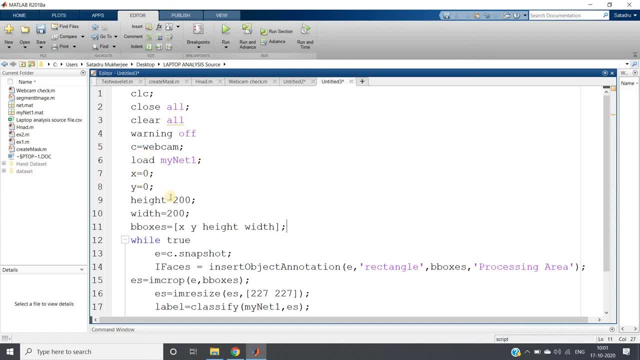 0. y equal to 0, that means from left top corner it will start, and height is 200. with this, 200, okay, while true infinite loop right, then e equal to c. dot snapshot. each time i am taking snapshot using webcam object and then i face a. 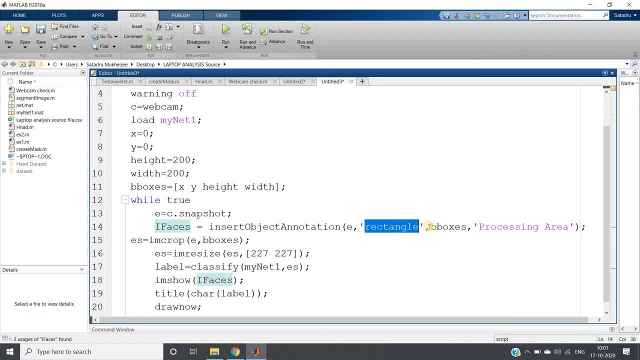 is equal to insert object annotation. e comma, rectangle b box is processing area. what it means: see here the processing area we have to highlight for that insert object annotation, that is, it will level one particular area of our interest. okay, e is our actual image. whatever our snapshot, it is taking the rectangular area we want to give and where that is b boxes. 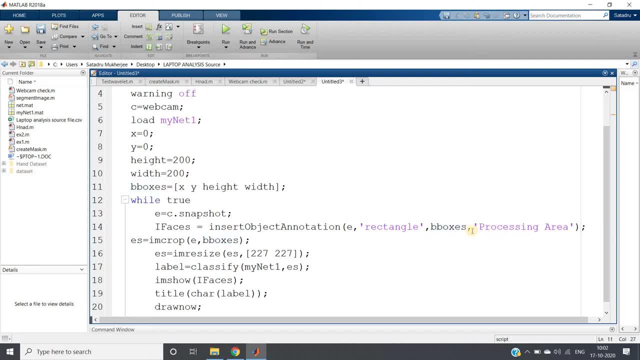 it is specifying in which part the particular processing area should present, and this is to give the name processing area. okay, nothing else there in that when i will show you the simulation, you will see that that particular area is highlighted and it will show processing area in below that. 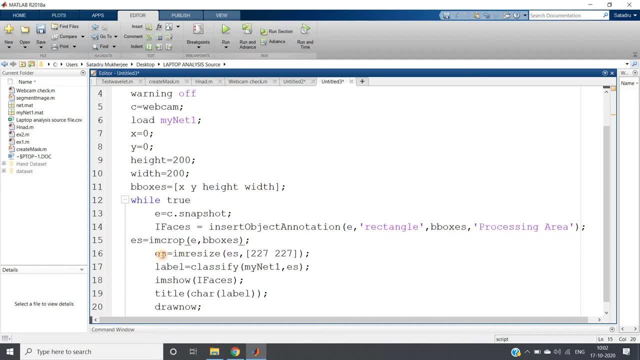 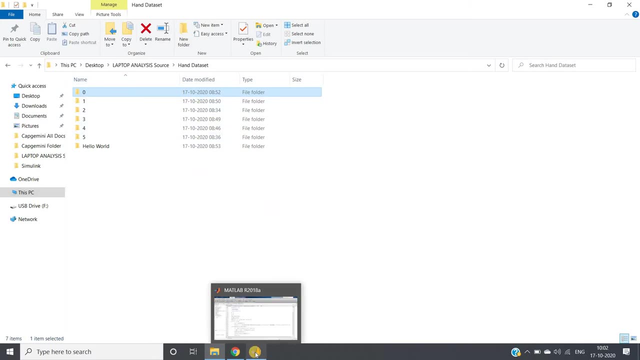 okay, then, cropping that particular part, only resizing that to 227 cross 227, because alex net takes only 227 cross 227 image, and all these images, whatever is present in my database, are basically resized to 227 cross 227. later i will be discussing how we have created the database. 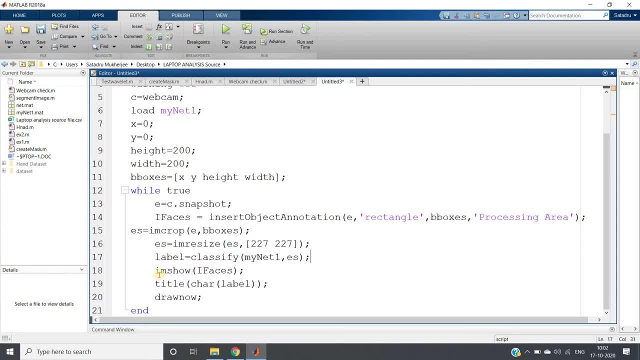 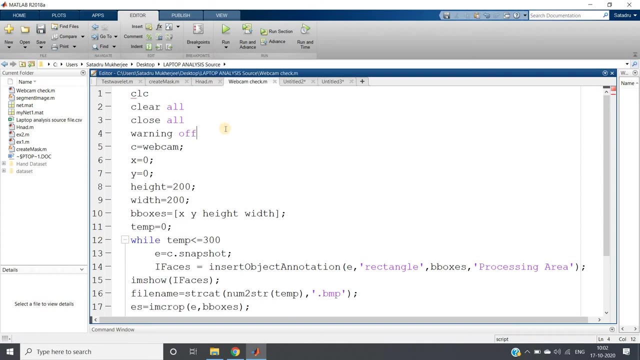 that time i will show you. okay, then we are classifying that and showing that and the classification output we are showing as title: okay, giving draw now for animation purpose. that's all, okay, and how i am, uh, creating the database. if you see the code, this is the code for creating. 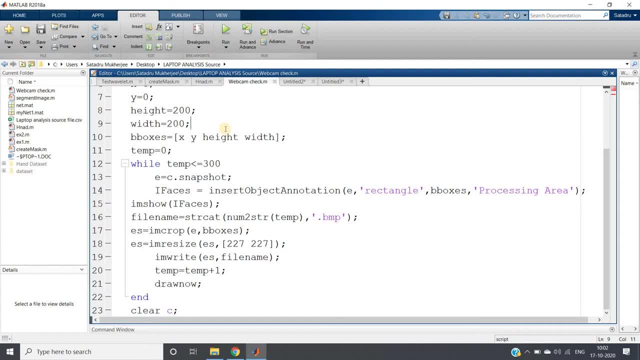 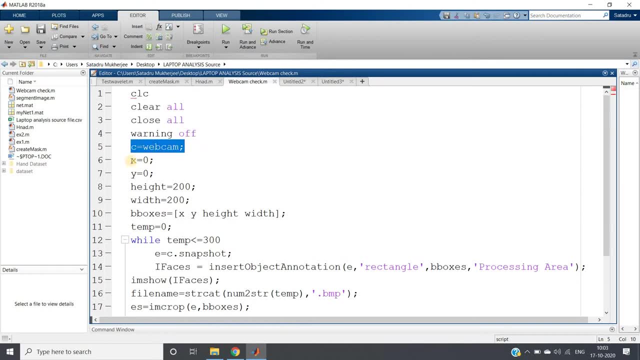 database. all the codes will be posted in the description box or in the comment section. okay, if you want, you can check their knowledge, dory. so see, here i am writing: clc, clear, causal c equal to webcam. okay, and again, defining the processing area and temp less than equal to 300. so 300 images for each class we are going to take. 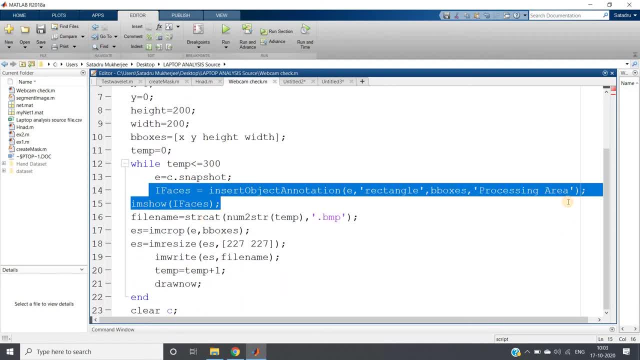 right. and then we are, uh, mentioning the processing area and showing that image, and then we have to store that in the database, right? so we have defined here temp equal to 0, one temp variable. it will store that with that temp. so temp will be initially. then we are incrementing temp here. it will be one next time it will be. 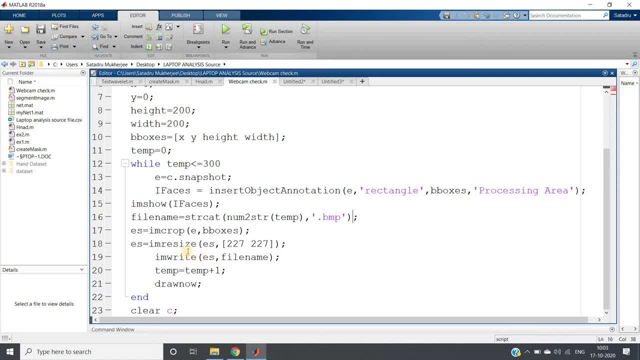 two next time like that, and dot bmp format: okay, but as our alex net takes only 227 cross 227 image, so i am resizing that. before that, we are cropping that particular region of interest and resizing that. and i am right, yes, uh, comma file name. okay, that's all so and at the end, clear c. 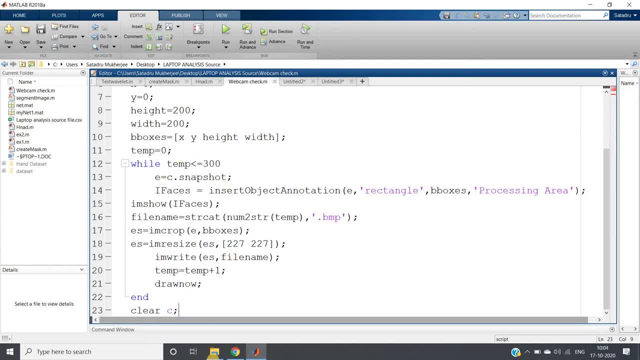 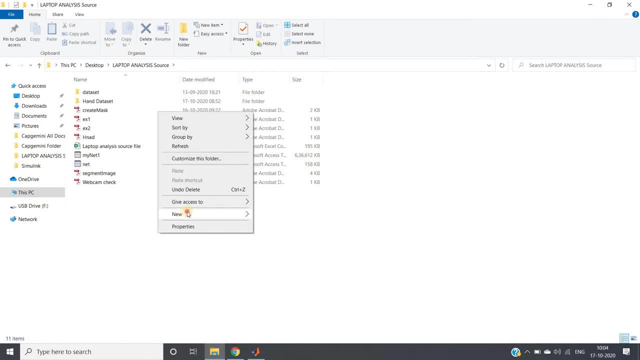 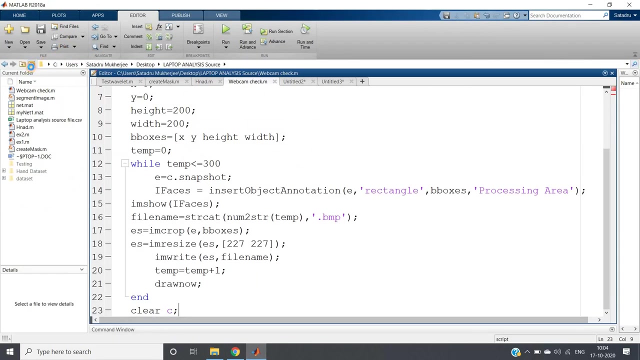 closing the webcam. so first let me show you one sample case: to create database. okay, so here, suppose, in laptop data analysis, i am creating one database, one folder. i am creating, suppose, folder name. i am giving randomly, okay, testing right now what we have to do. we have to first take the directory, current directory, to testing. 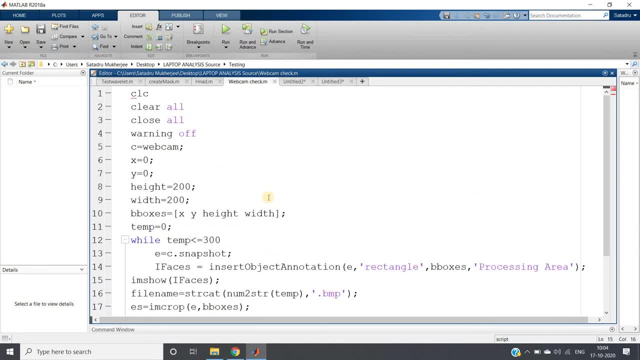 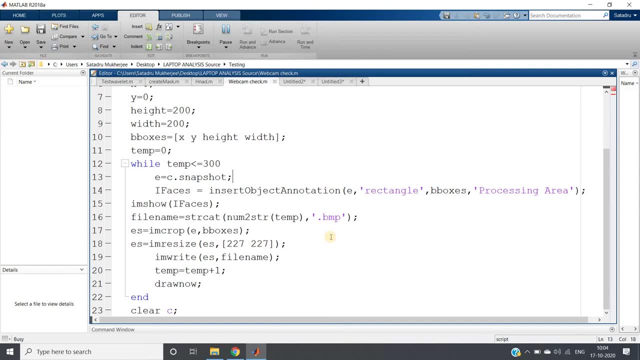 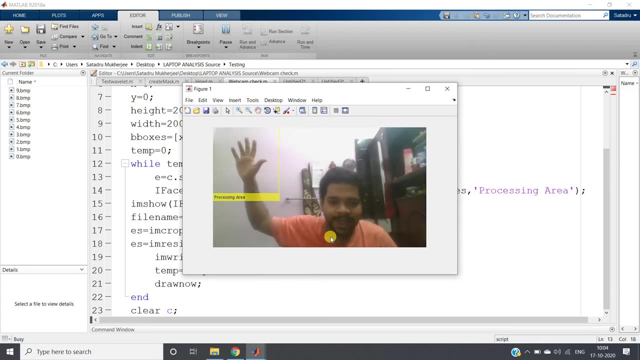 i will double click on that and select folder okay, and then i will click here, right then, if i run this particular part, you can see one image will open and one processing area will come. see, processing area came here. i will take my hand and it will capture only this. 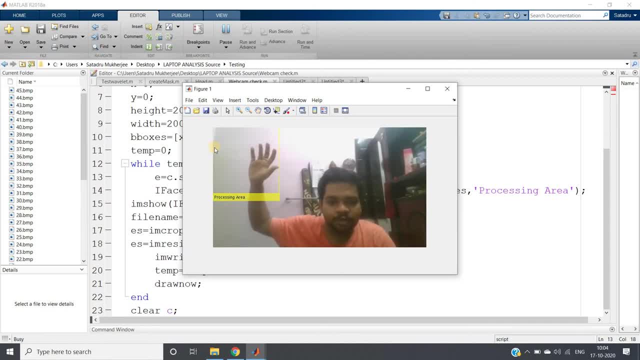 particular part and it will resize this particular part to 227, cross 227. it will be capturing 300 images and store in this directory testing. okay, so later we can. if we want, we can use this particular part. like here i can make this particular part. like here i can make this particular part. like here i can make. 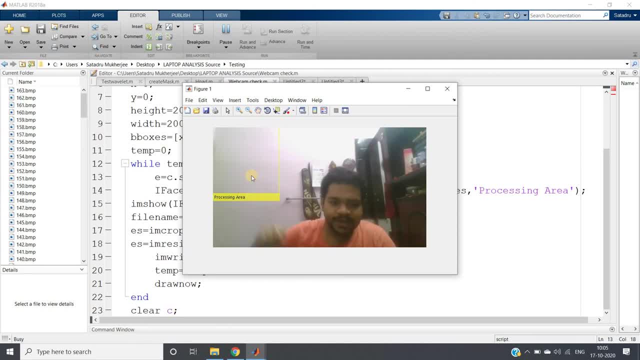 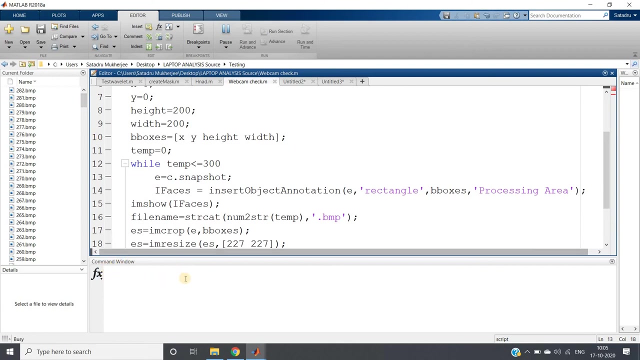 so this is going to take 300 images. okay, and this particular part it will not consider right. so this is how you can create your own uh data storage. okay for classification. so it is going to complete. as soon as it will complete here, double angular bracket will come, so let's wait for some time. see this completed. it has taken 300 images. now, if i go, 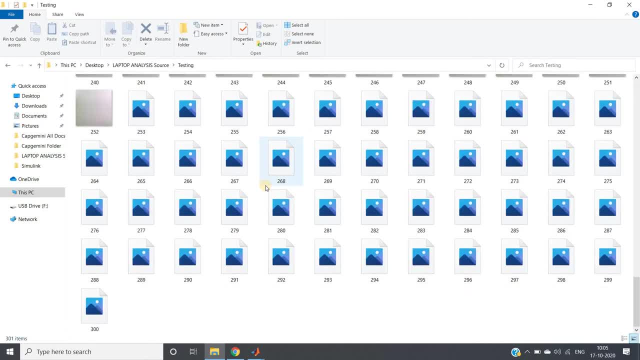 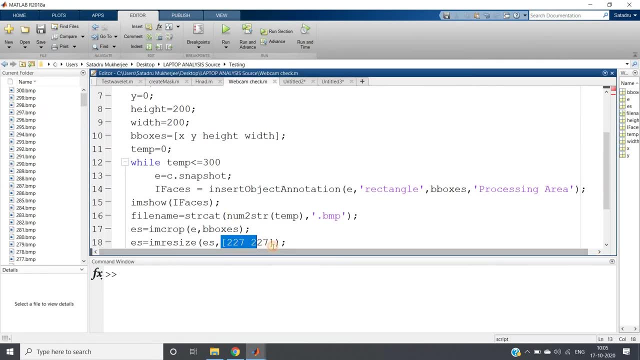 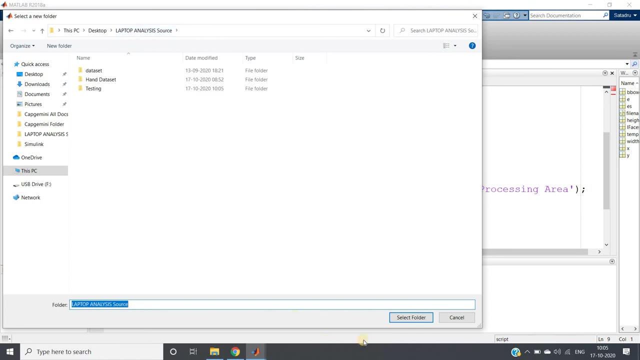 go to testing. see here the 300 images, each of size, how much 227 cross 227 is stored, because you can see that we are resizing to 227 cross 227, like that. okay, so this is how we are creating the database. i hope you can understand simply. now i will go to again my original directory, where my 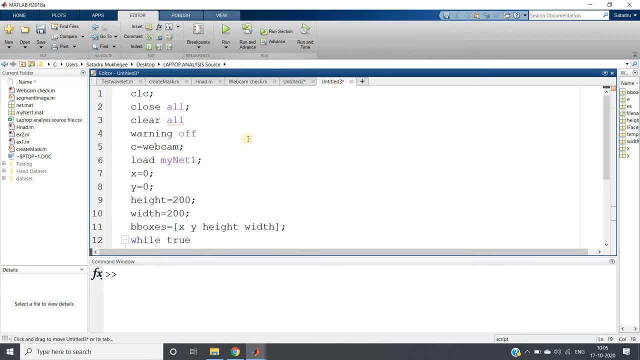 mynetmat is stored. now i will run the main testing code, which is this one: okay, so ctrl a evaluate selection. so it will take some time to load the model, whatever we have trained earlier. okay, and here it goes. it is taking some time because you can understand, the data set is quite huge, right? so that's why.